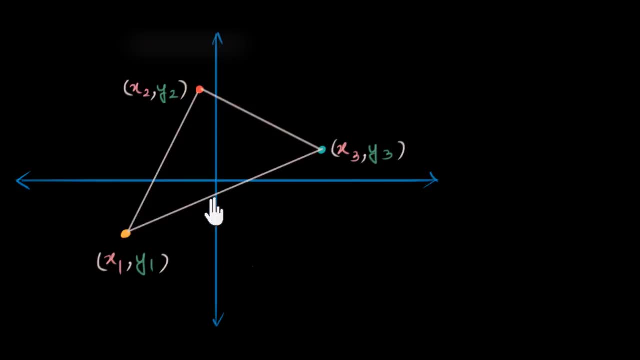 lengths of each of these sides. That was the second thing that struck me. Maybe I can find this length, this length and this length, and then use Hiron's formula- I don't know if you remember it, because it's that root of s- into s minus a, into s minus b, into s minus c formula. You can use that. 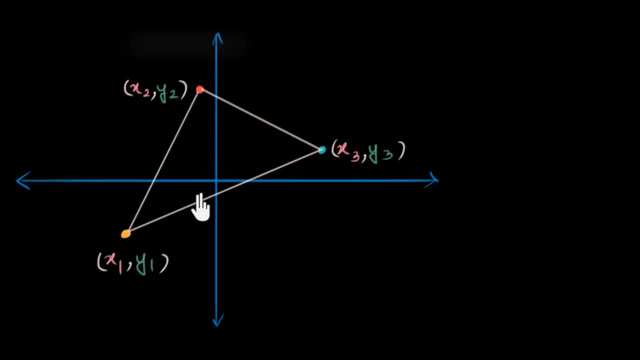 and then you can find the area of this triangle. That will definitely work. I encourage you to try it. I just did the calculations and looked so big that I was just gonna. I realized that is probably not what this question's trying to get us to do, which is to find the area of this triangle. 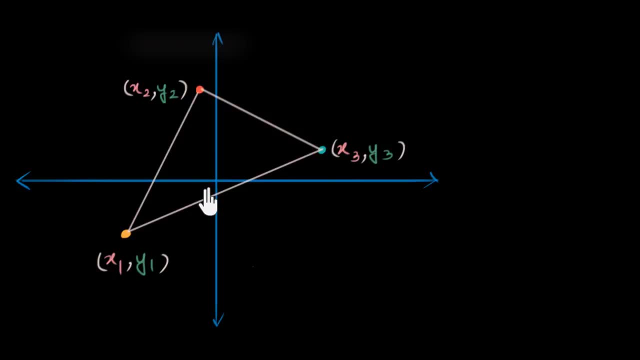 in somewhat a simple way. So if both of those are not possible, then what can you think of? The thing about coordinate geometry is that it gives you all the lengths either horizontally or vertically, And the problem here is that we don't have any of these lines being horizontal or 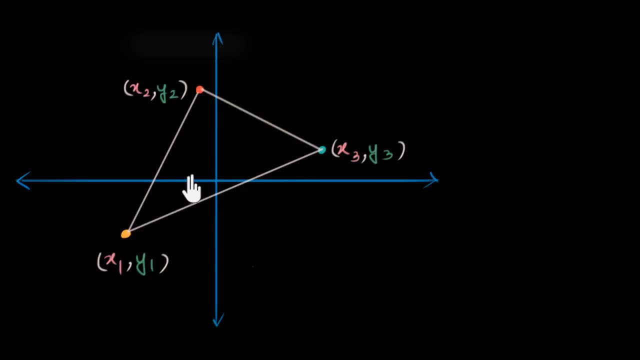 vertical. That's what makes the triangle is just long and it's a bit of a hard to see. It's probably this question not directly easy. So then, what can we do? I want you to stop right now and think: can you express the area of this triangle? 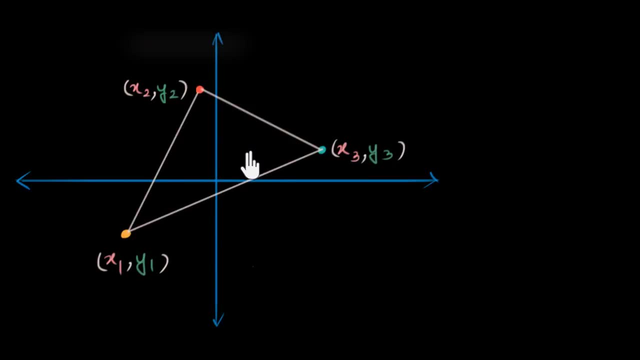 as some figures, some triangles or rectangles or something such that all of them have only vertical or horizontal sides. Can you think of that? Now, when I can't think of something, I'm just gonna start drawing some vertical and horizontal lines and see where it leads me. 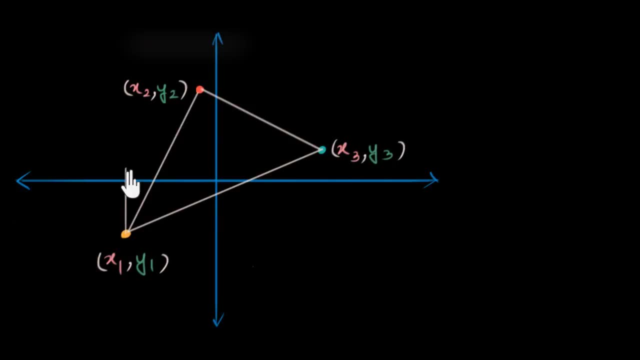 Maybe I'll get lucky. Let us see, I'm gonna draw a vertical line from here and then maybe a horizontal line from here, and I can begin to see some pattern that I can form here. So if I connect these two, I see a triangle here. 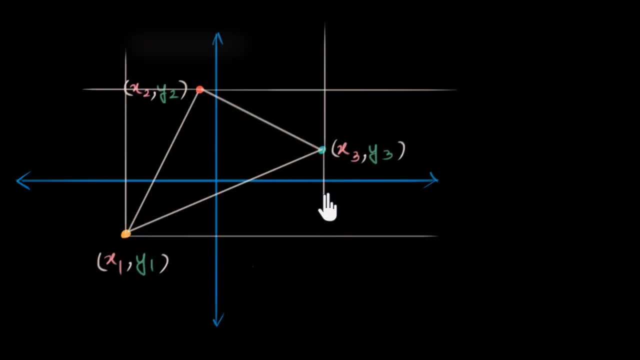 Then maybe I draw some more here, another one there, another one here, And now, finally, I'm able to see there it is. Can you see it? There is a rectangle over here which covers this entire region and there are these three triangles. 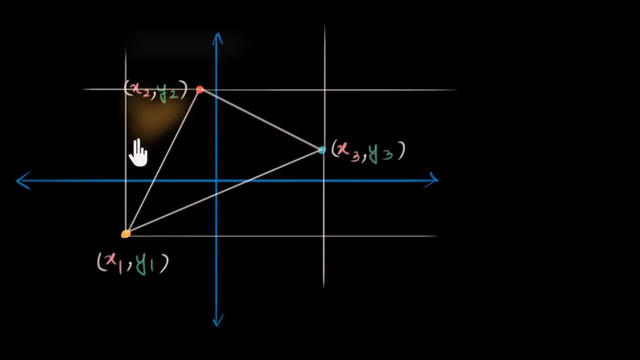 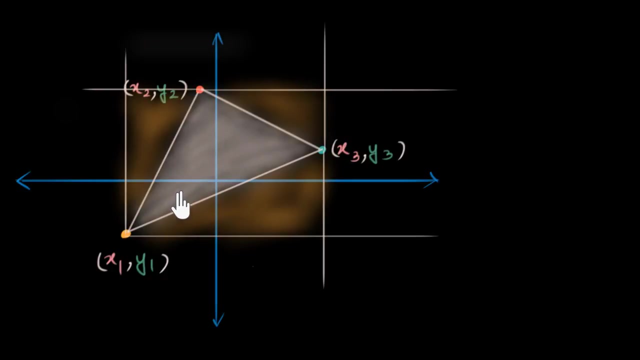 So let me shade these triangles, Triangles. I have these three triangles whose area, if I subtract from the original rectangle this big one over here, I will get what I want, which is the area of my triangle. So I actually have my path ready. 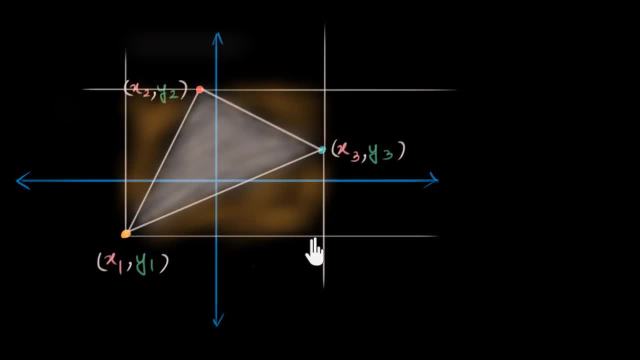 This should work, because my rectangle has only horizontal and vertical lines in it, and my triangles have both. all of them have a base and a height that is either vertical and that's vertical and horizontal. So my job is done. Now my job is to find the lengths of these. 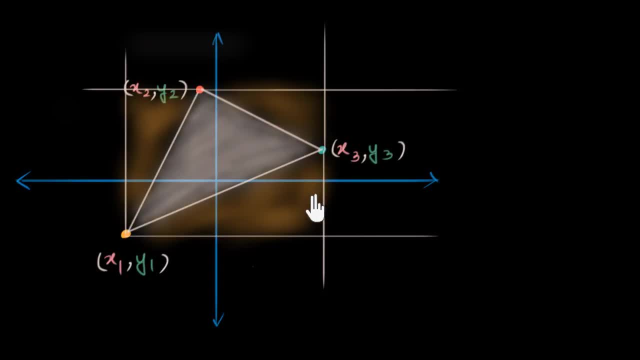 so that I can proceed and finding the lengths in coordinates. geometry for horizontal and vertical is usually direct, So let's do it. So let me first find this big side of the rectangle, So that's gonna be this entire side, And what is that equal to? 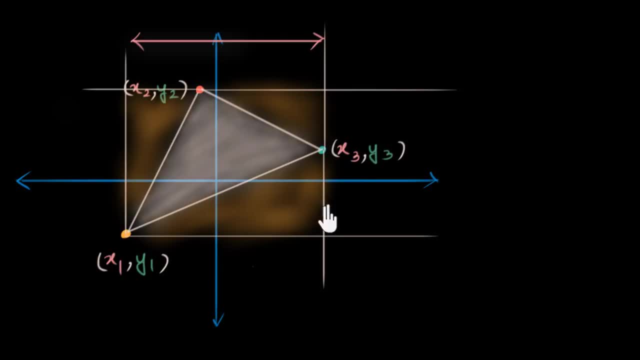 You can see that the x coordinate of this line is x3.. I'm saying this line because all points on this line will have the x coordinate x3 and all points on this line will have the x coordinate x3. In other words, this length is x3 minus x1. 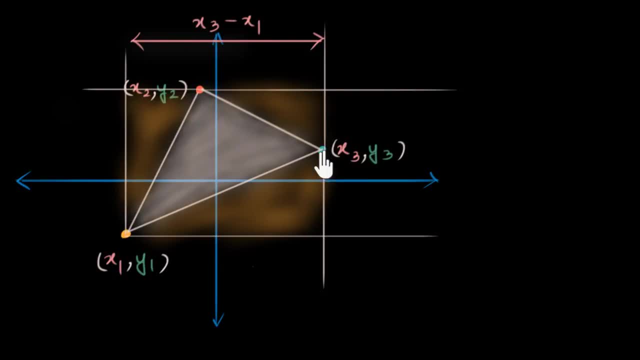 X3 minus x1.. And the next thing I'll need is the y coordinate, this big line over here. So what is that gonna be equal to? Similar story: y2 minus y1.. Y2 minus y1.. All the points over here have the y coordinate, y2.. 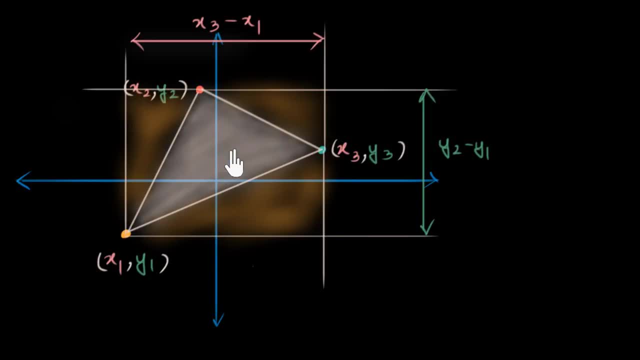 All the points here have the y coordinate y1.. You can do something similar. It's a similar story for all points over here. All of these other sides we need. What other sides do we need? I need this so that I can find the area of this triangle. 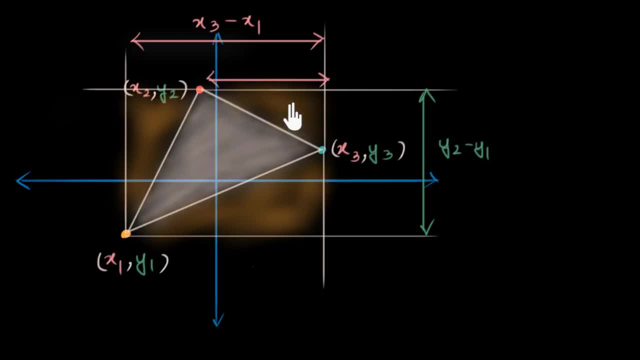 So what is that gonna be? That's going to be equal to x3 minus x2.. X3 minus x2.. This one here I will need, That is x2 minus x1.. X2 minus x1.. I will also need this one. 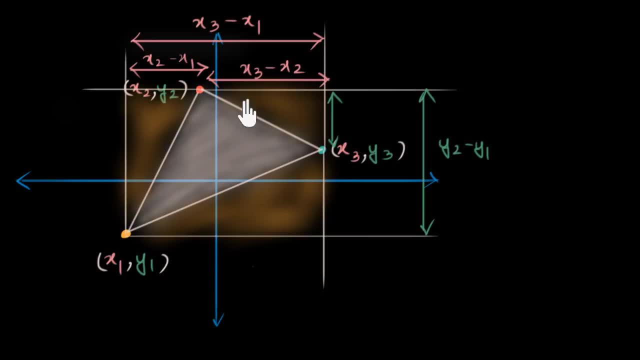 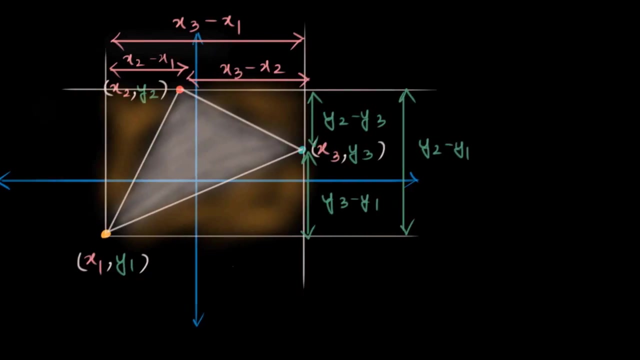 This y coordinate, That is y2 minus y3.. Y2 minus y3.. And I will finally need this one, Which is y3 minus y1.. Y3 minus y1.. The diagram looks a little bit cluttered, but we have everything we need. 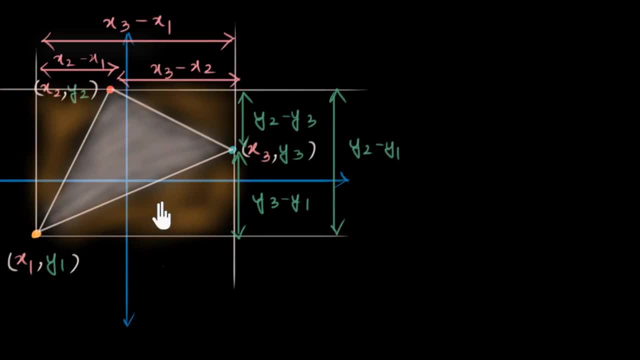 So what is our next step from here? Our next step from here is to write the area of the rectangle down first. What's the area of the rectangle? It's length into breadth, or x3 minus x1, multiplied by y2 minus y1.. 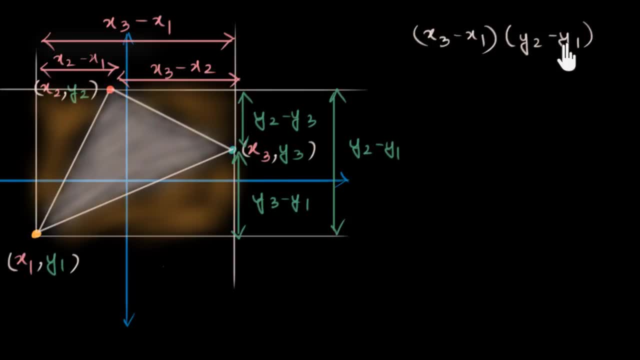 Y2 minus y1.. Y2 minus y1.. This is the area of the rectangle. Now I need to subtract the areas of each of these triangles. Let me start with this one. So let's say I do minus half into base, into height, right. 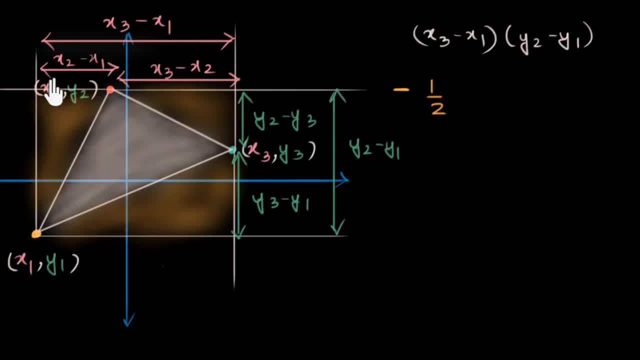 So half into base, Let me just take. I can take whichever I want as the base. So base is: let me take x2 minus x1.. X2 minus x1 multiplied by height, In this case that's y2 minus y1.. 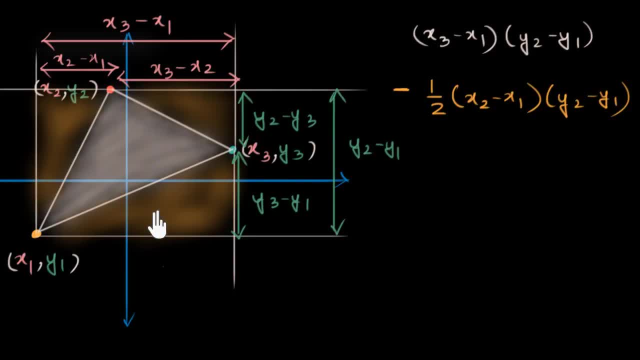 Two minus y1.. And now I will subtract, say this triangle Minus half into. for this triangle, the base is x3 minus x1.. X3 minus x1.. And the height is y3 minus y1.. Y3 minus y1.. 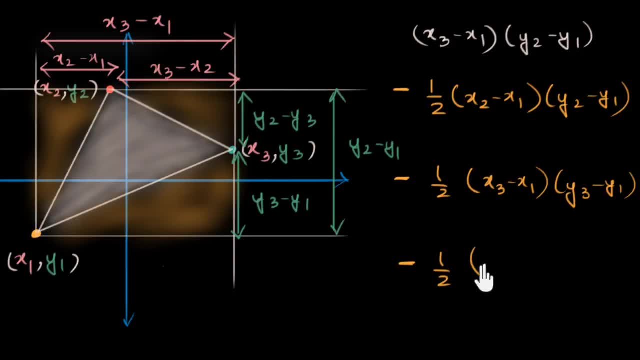 And finally the last triangle over here. so it's one by two into minus half, into base Base: x3 minus x2.. X3 minus x2 into height: Y2 minus y3.. Y2 minus y3.. Now r. 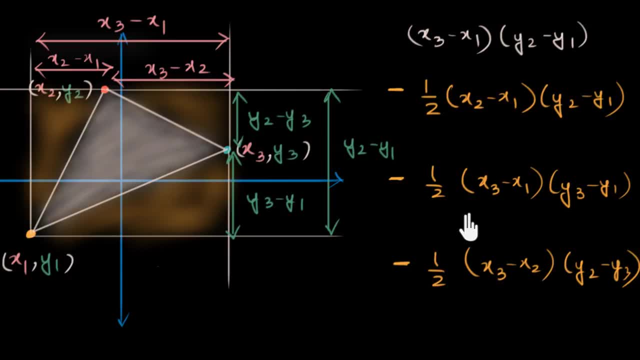 Let me just move this little bit over here. yeah, So now our job actually is to simplify this, And the thing here is that, even though this doesn't look too beautiful, the final result we get when we simplify a lot of terms: cancel. 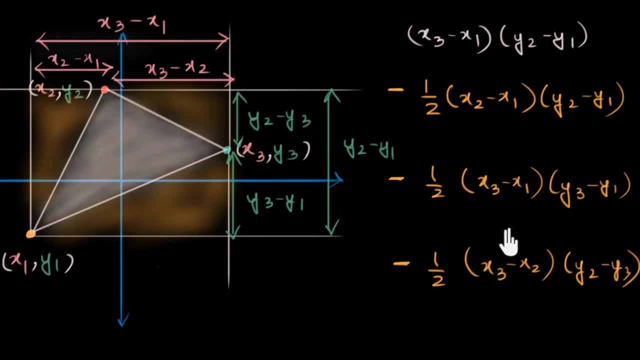 So the thing you get looks pretty beautiful, actually, Like I was surprised when I first saw it. So pause this video right now and watch what happens when you expand all of these terms and look at what cancel and look at what the final result you get is. 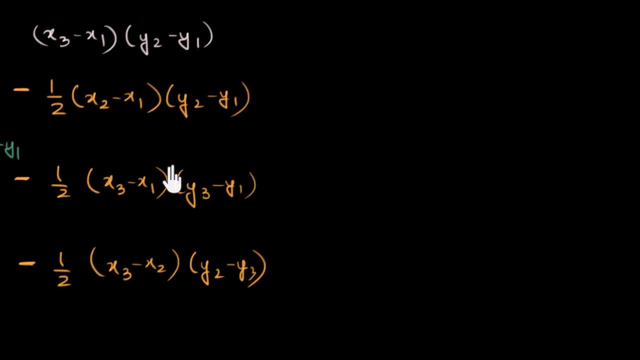 I'm gonna do it now. I actually don't need the diagram anymore. I only have to simplify this. I can look at the diagram later. So one thing I'm gonna do first is I'm gonna take this half outside. You know, I don't wanna keep dealing with halves. 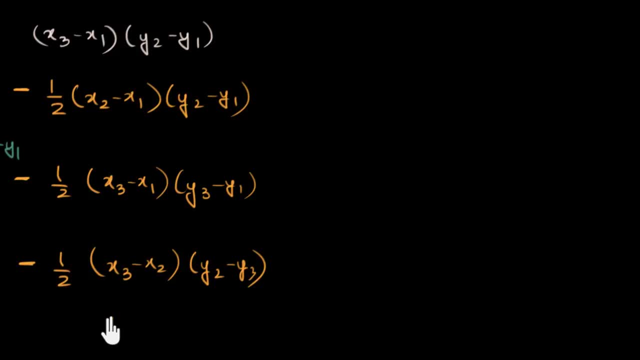 I really don't like that, So I'm gonna take the half outside. So I know my answer's gonna have a half outside, which means that I can now start simplifying each of these. I'm gonna do it in each of these, in one line. 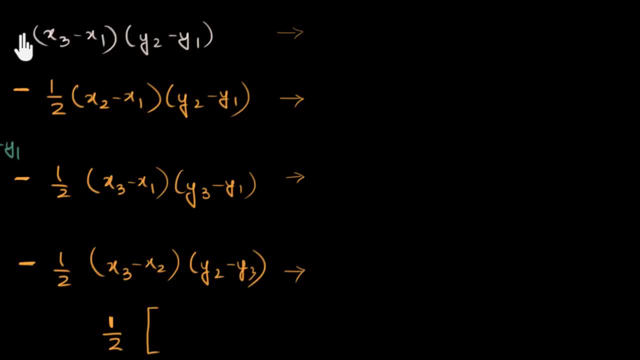 and then let's look at what we get. So I'm gonna put a two over here So that I have. I've forgotten these halves and I added a two over here. I know I'll have a half outside. So what is this gonna be? 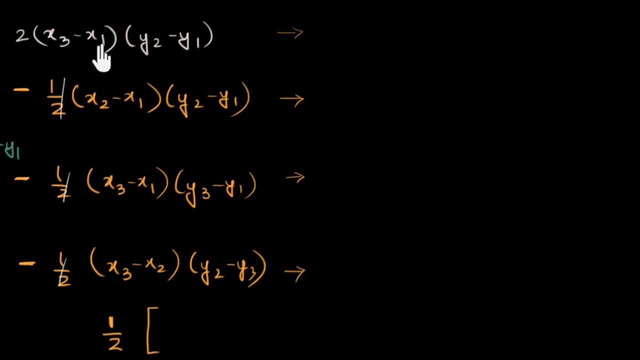 Now the way I like to think about such things is I get very confused when I do signs and this, two and all that. So I'll first look at the terms, then I'll add the signs. So I'm gonna have x, three, y, two. 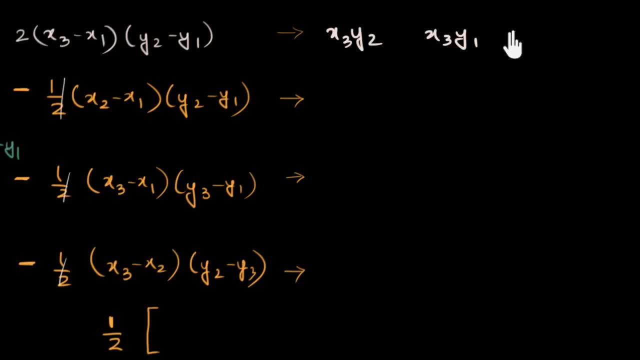 x three y two. x three y one. x one y two and x one y one. I know these are gonna be my four terms. Now I can figure out my our signs. So all of them are gonna have a two. 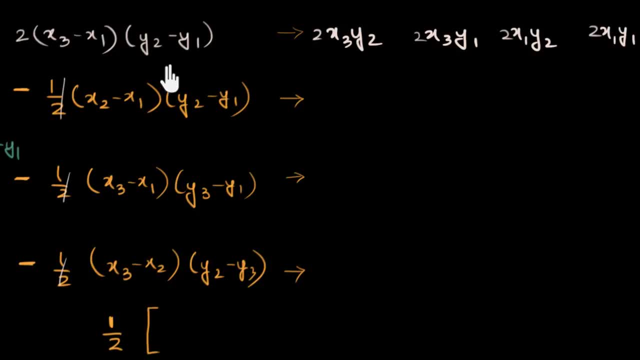 So I know that all of them are gonna have a, two and I know that the middle two terms are gonna be negative because it's a minus b, right, And these two are gonna be positive. So two x three y, two minus minus and finally a plus. 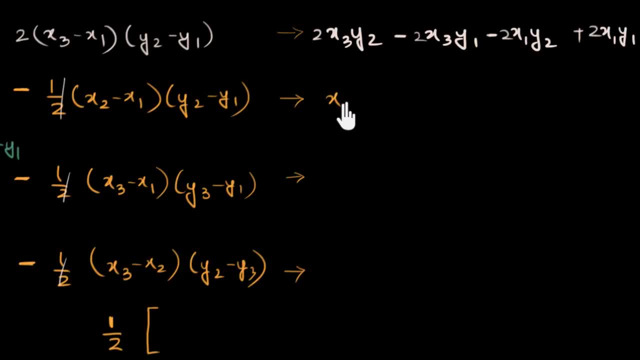 So then I'm gonna do this. Similarly, I'm gonna say: x two y two is gonna be the first term. X two y one is the second term. X one y two is the third term. One y one is the last term. 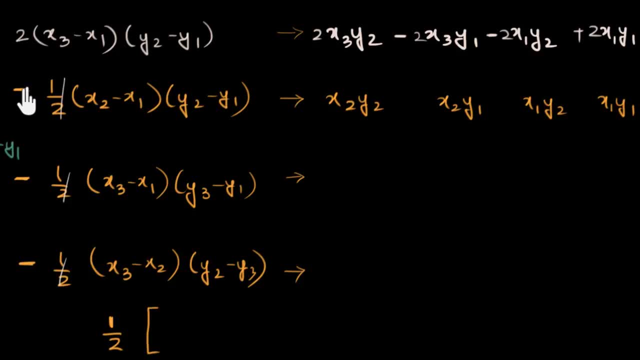 Now I'll figure out the signs. There's a negative outside. Oh, I hate it when that happens. That's where I make most mistakes. So what I'm gonna do is I'm gonna add negative here. This would have been negative. 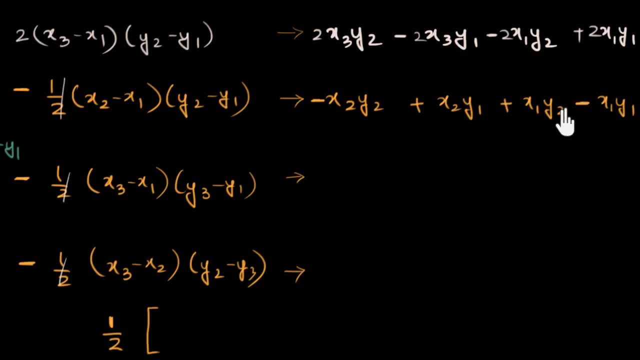 so this is positive here, positive here and negative here. I'm gonna keep the same pattern going so that I know it's gonna be minus plus, plus, minus. So I don't have to think about it at all. Think about it at all. 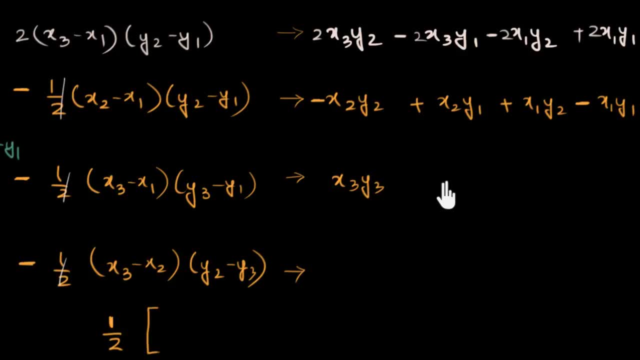 That's what I wanted to say. So x three y three x one. Let me X three, y one, X three y one, X one, y three And x one, y one. There it is, And again it's gonna be minus, plus, plus, minus. 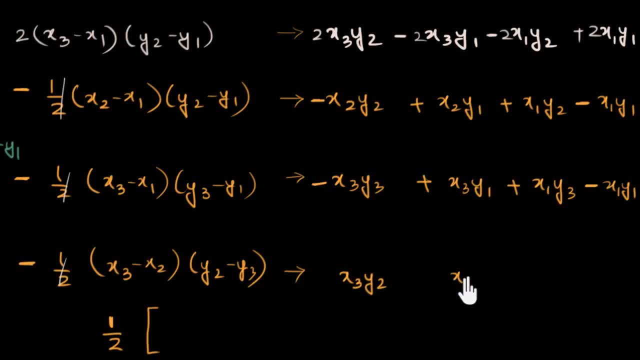 Similar story here: X three y two, X two. Sorry, x three y three, X three y three, X two y two And x two y three. Need to move this a little bit so that we can see that. 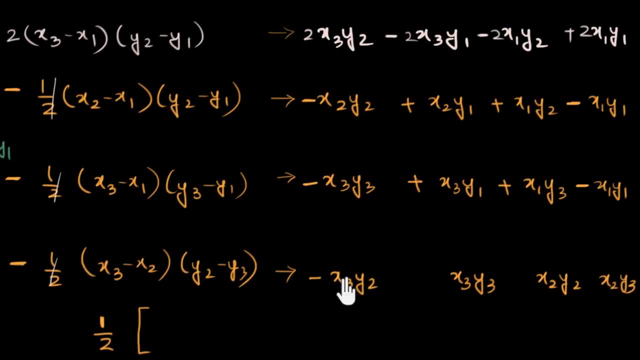 Yeah, X, two, y, three, And again it's minus plus, plus minus. Now our job is to start canceling out, because we know something's gonna cancel out. This expression's really large, so we've seen that. the final expression. 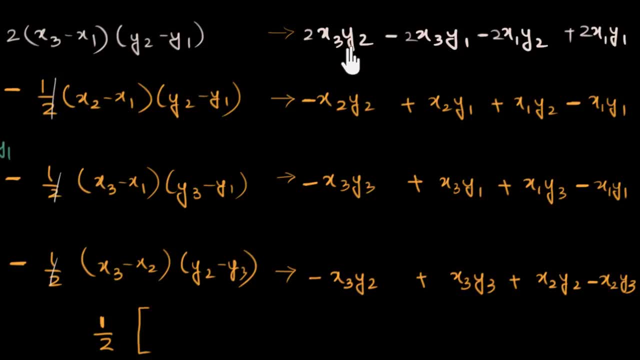 is actually quite smaller than this. So let me first see X three y two. Can I find x three y twos here? I can find one here. So this two goes away and this entire expression goes away. X three y one: I can see one over here. 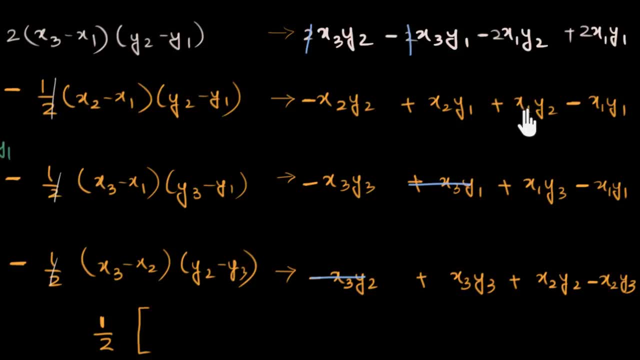 So this goes away and this two goes away: X one y two. I can see plus over here. This is minus, so this one goes away Plus two x one y one. I can find one x one y one over here. 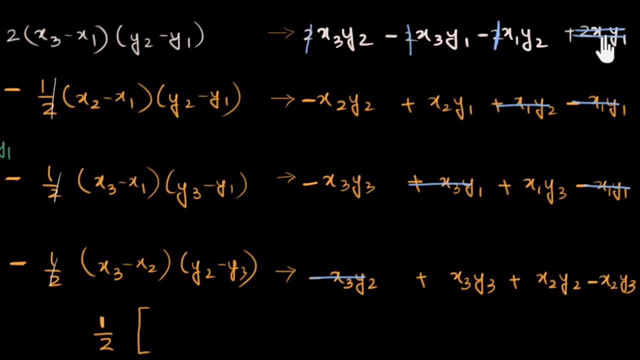 and I can actually find one more- x one, y one over here. So, oh, this entire thing goes away. I like it when things start getting canceled like this. Let me see if there's anything else: X two, y two. 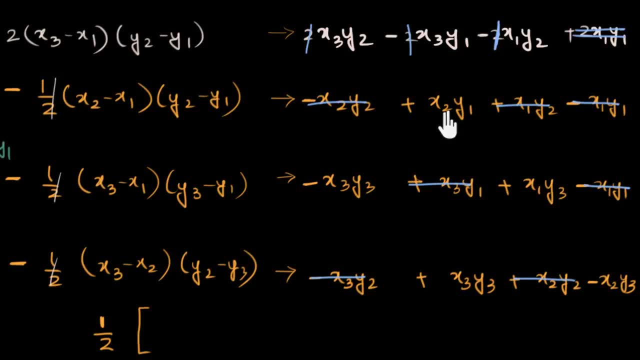 X two y two- Okay, I can see one here and a positive one over here. X two y one. I can't, Can't see anything. X three y three. I can see one over here. This goes. 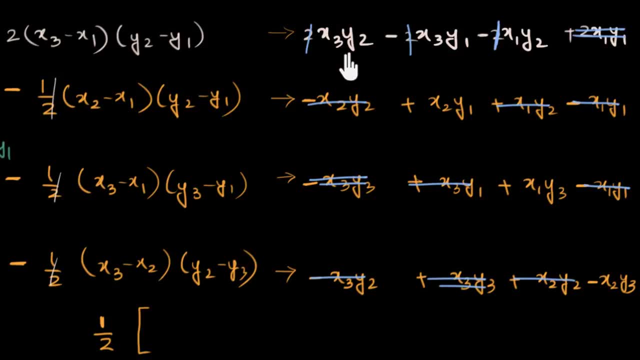 So finally, it looks like nothing else will go. So how many terms do I have? One, two, three, four, five and six. So these six terms are gonna be there in my final expression, but if you notice, it's actually much simpler than what we started with. 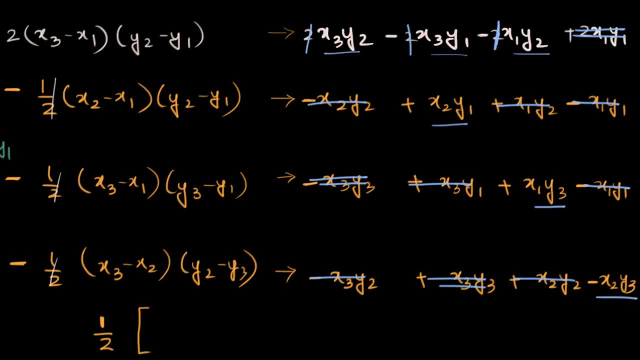 So I'm gonna start writing this expression now. So I'm gonna take the x is common, because I can see that there is an x three y two here, x three y one and so on. So x one y three is there. 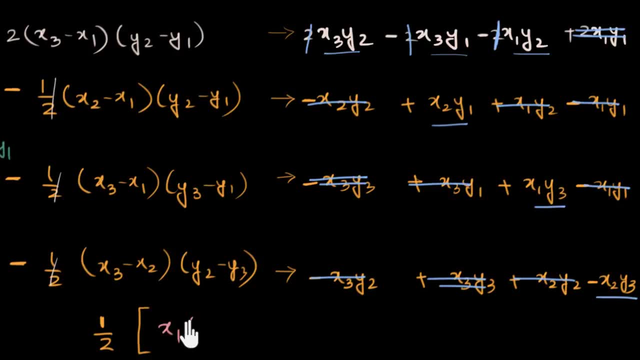 X one, y two is there, So I can take x one common and write it X one into. so it's not like there's a big reason I'm doing it. it's just that I find that the final expression looks more beautiful. 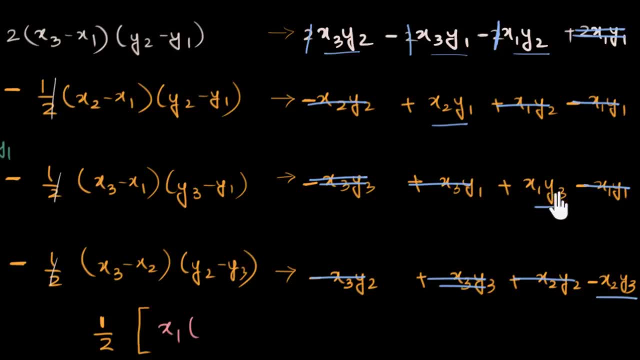 when we do it like this: So x one into what? Y three minus y two, Y three minus y two. Now, what is the next one? I'll take x two common out over here, And then I'll have, if I take x two common. 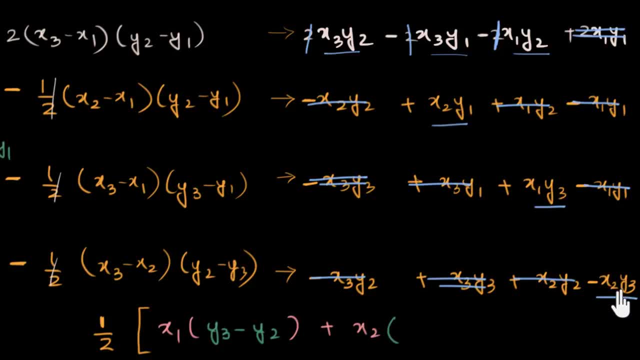 I'll get x two, y one minus- ah, it's here Minus y three, so y one minus y three. Y one minus y three Plus. I'll take x three common now and I will get y two minus. 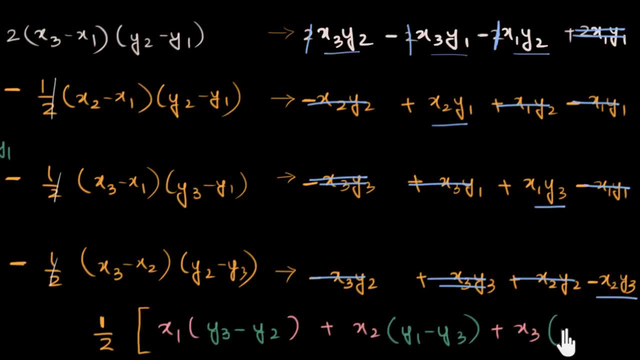 y two minus. oh, it's here: Y two minus y one, Y two minus y one. And there we have it. Now. I don't know about you when I see this, but I'm amazed that what we're getting here. 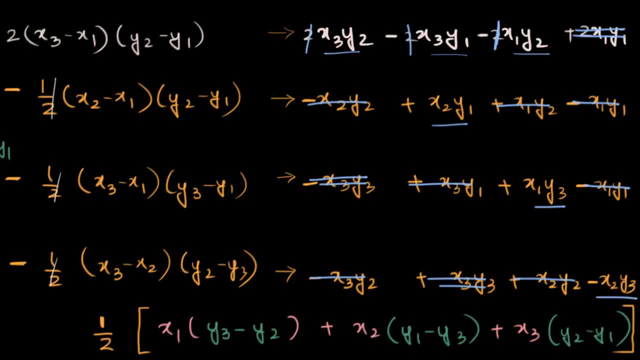 is so much simpler compared to like what we get when we do the Heron's formula or any of those things. It's basically just the first coordinate, one of the x coordinates, the difference of the other two plus the second one, one minus three.